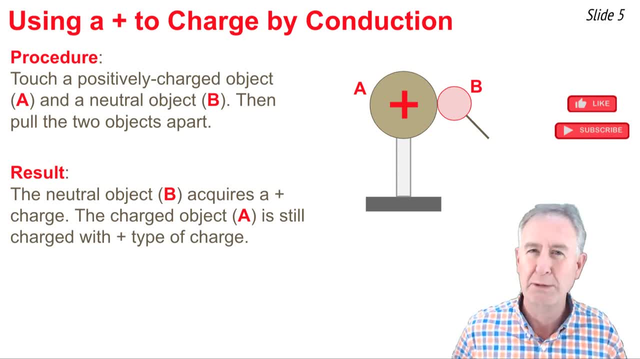 how do we explain this? There's two very common incorrect explanations that we really need to be careful about, And the first one is the explanation that object A transferred positive protons to object B, And that's incorrect, because protons are bound up in the nucleus of the atoms and 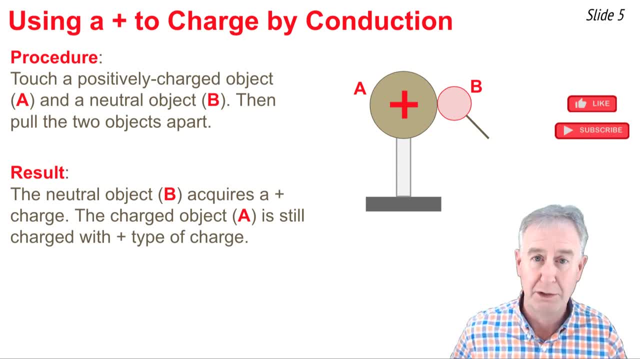 incapable of being transferred from one object to another by an electrostatic event. It would take a nuclear event to split that nucleus open and get those protons out for transfer. That doesn't happen by touching two conductors together, So that's the wrong explanation. The 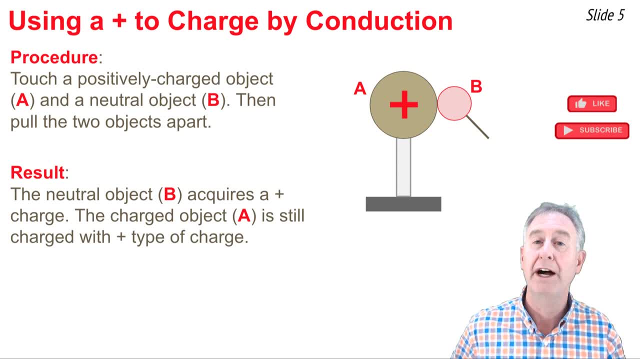 second wrong explanation goes like this: Object A transferred positive electrons to object B, and that's a no-no as well. So what is the right explanation? Well, it has to involve electrons, and electrons are negative. So let's think a little bit about object A and object B. 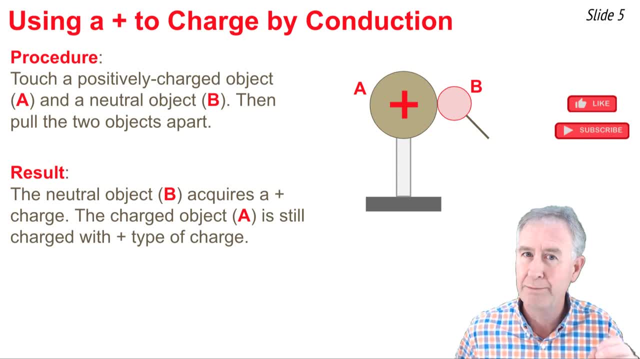 Object A is positive, so it has protons. it has electrons, but more of the protons than the electrons. You might say it's short on electrons. And then object B is not short on electrons, neutral, So it has protons. it has electrons and equal numbers. Now some of the electrons in 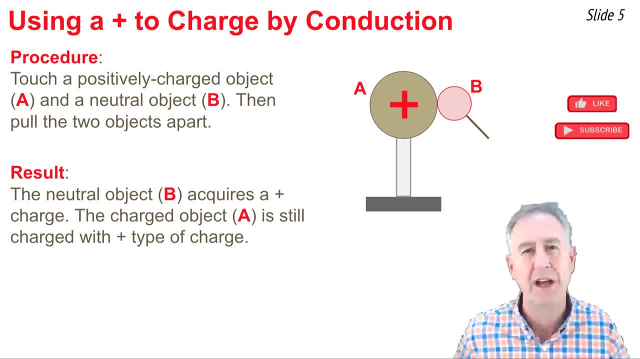 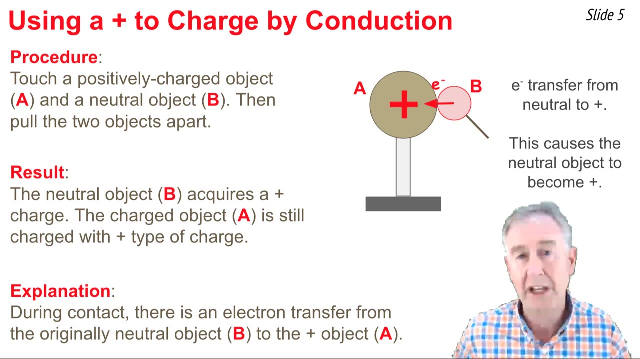 object B, when touched to object A, notice a positive charge And electrons love positive, And so some- not all- of the electrons in object B migrate onto A, being attracted by the positive charge, and there's a transfer of electrons from B to A When a neutral object loses electrons. 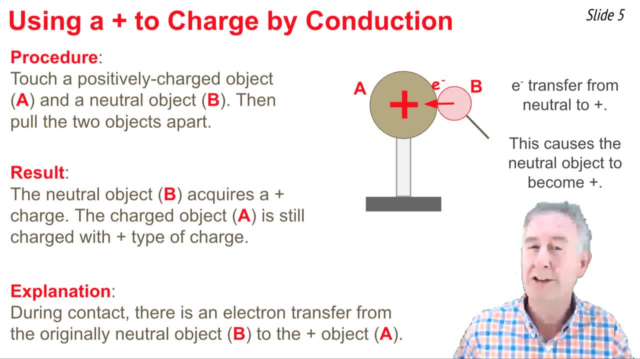 it becomes positive. So object B is positive, And when a positively charged object gains some electrons it's positive, And when a neutral object loses electrons it can gain some electrons. amount of positive charge it has will decrease, And so that explanation is perfectly consistent. 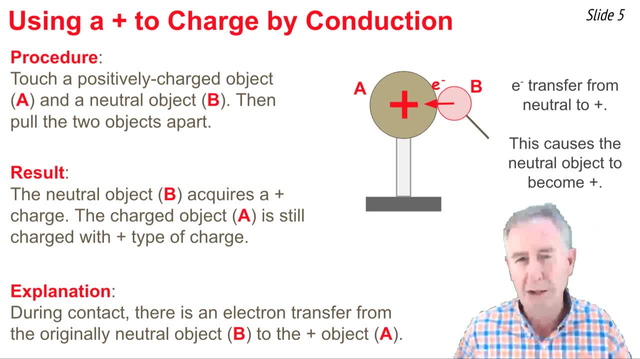 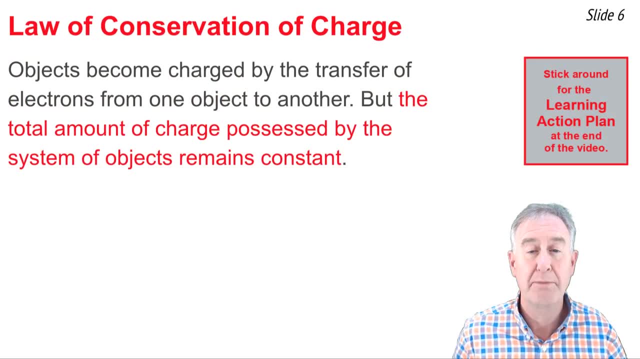 with the observations of what the result is, and it follows our rules about the nature of electrons and protons. Now, like all of our charging methods, the charging by conduction method follows the law of conservation of charge, which states that objects become charged by the 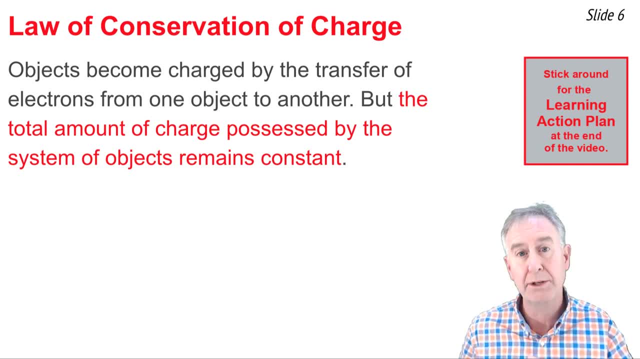 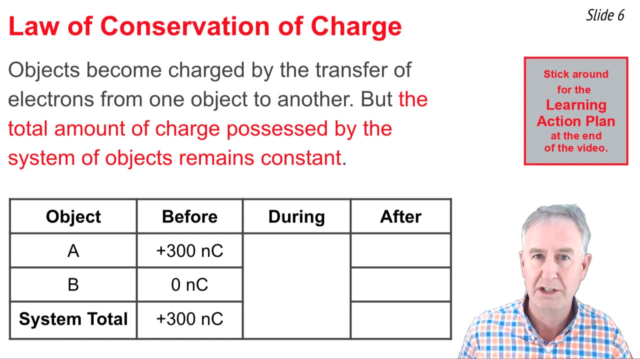 transfer of electrons, but the total amount of charge possessed by the objects combined by the system of two involved objects remains constant or unchanged. To illustrate this, let's consider that last example we discussed, where you charge by conduction a neutral object using a positive. 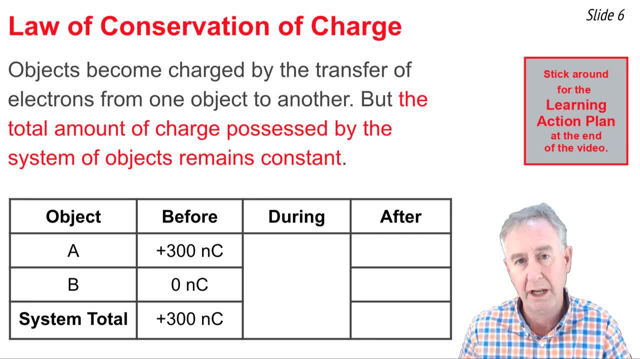 object. So here's a table and we see columns of before, during and after in rows of object A, the positive object, object B, the neutral object, and then in the bottom row is the system total. So before the actual process begins, object A has 300 units of charge, positive 300.. The unit there is the charge, So object B has 300 units of charge positive 300.. So object A has 300 units of charge positive 300.. The unit: there is the charge, So object A has 300 units of charge positive 300.. 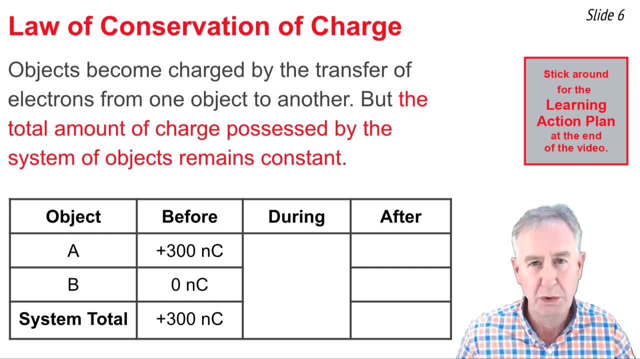 There's nanocoulombs- We'll just refer to it as unit- And object B is neutral, so zero, And the system total is positive 300 units of charge for the two objects combined. Now, during the process, object B transfers electrons to A And, as we mentioned, when object B loses electrons, it 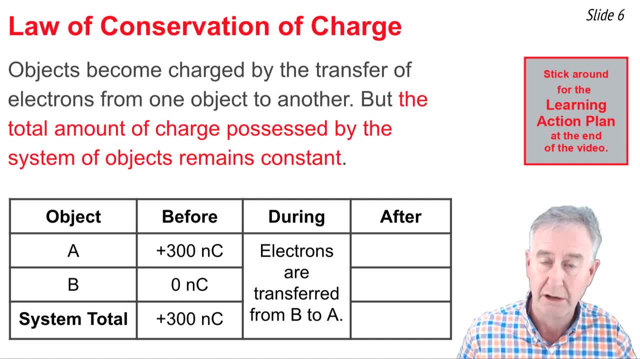 becomes positive And when object A gains those electrons, its amount of positive charge will go down. So we just need to make up a number here. I'm going to make up 100.. 100 units of positive charge are lost from, or I should say 100 units of negative charge are transferred from B to A. 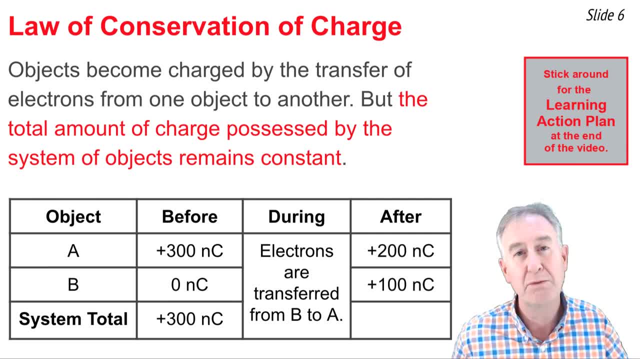 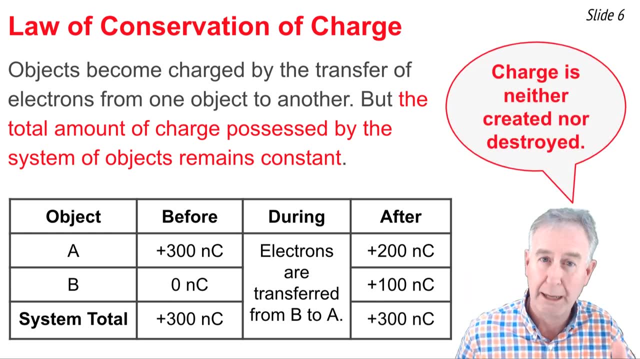 which makes that neutral B now have positive 100 units of charge And because object A has gained this negative 100 units of charge that B lost, A is going to go from 300 down to 200. And if you sum it up, the total amount of charge for object A plus B for the so-called system- is positive 300. 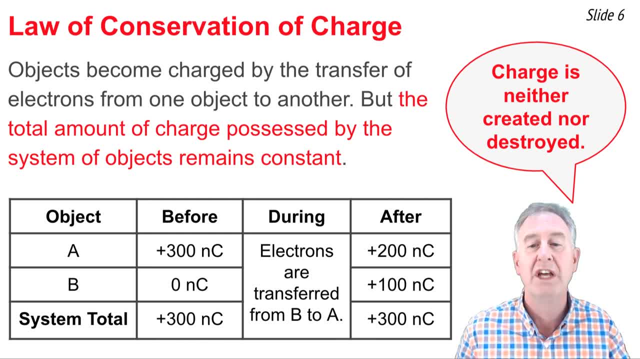 units of charge. So if you check the bottom row, you see that the total amount of charge for object A, you see the law of conservation of charge, that the total amount of charge possessed by the system remains unchanged or is constant. One way we sometimes put this is that charge is neither 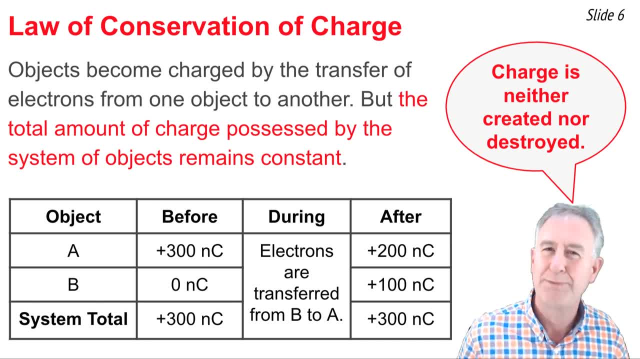 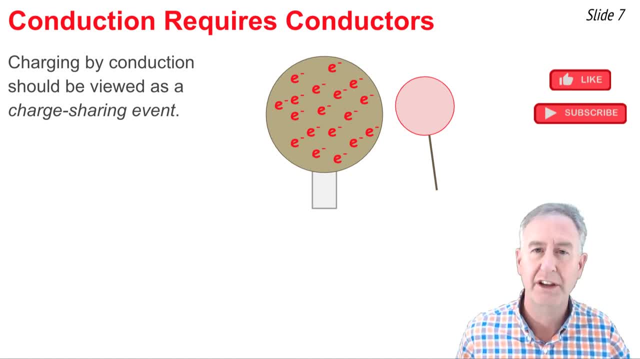 created nor destroyed, but only transferred from one object to another object. The way I like to get students to perceive of charging by conduction is to perceive it as a charge-sharing event When you make contact between the two objects. what is really going on is the objects are. 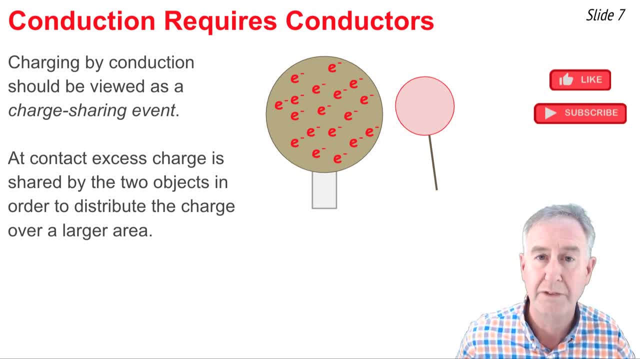 sharing their excess charge, It distributes over the surface of the two objects. So when we look at object A, the one on the left, the larger one, it has an excess of electrons, It has a negative charge. Object B, the neutral one, the smaller one, is going to touch it here. 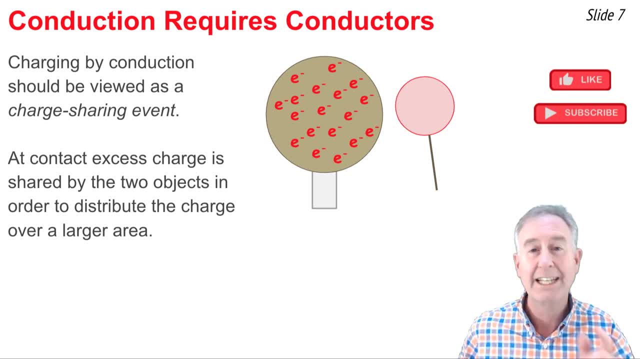 And when it does, electrons can move from object A to object B. So there you see it. I'm going to do it again. I'll go back and forth. You see it, You don't see it, You see it, You don't see it. 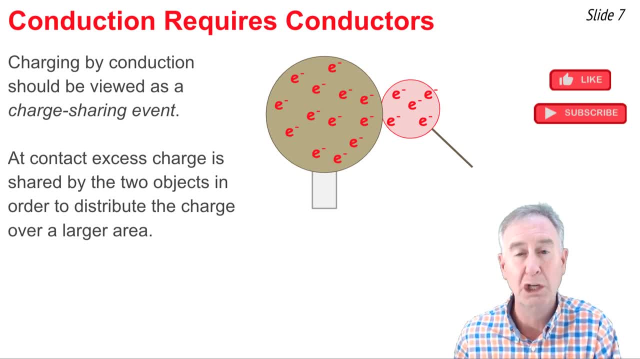 And what's going on up on contact is that you're not gaining or losing electrons, You're just sharing them. Object A is sharing the excess of electrons with object B. It's a charge-sharing event. Now, in order for this to occur, electrons have to be able to move. 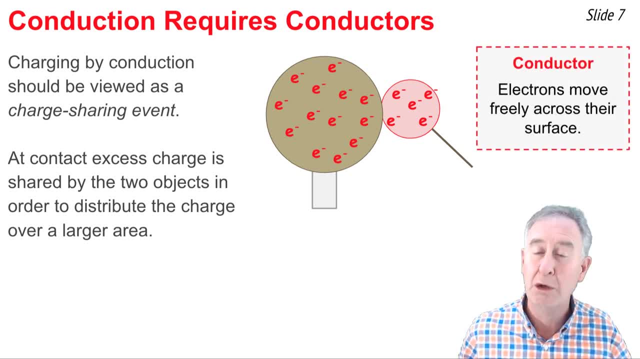 from A to B and across the surface between A and B, in order to distribute themselves evenly about the larger surface area. And that would never happen with insulators. Only conductors allow for the free flow of electrons across their surface, And so that's why we say charging by. 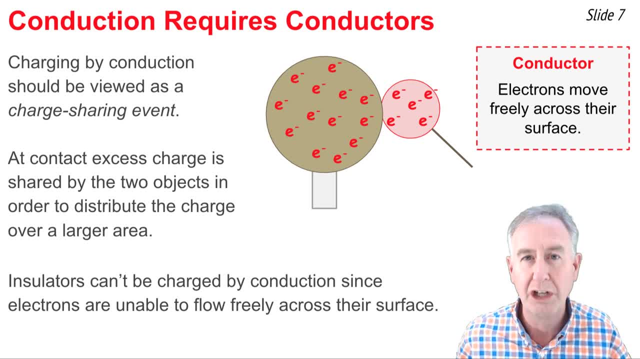 conduction requires conductors. Insulators can't be charged by conductors because insulators prevent the free flow of electrons across their surface, And so that's why we say charging by conduction requires conductors. Insulators can't be charged by conductors because insulators prevent the free flow. 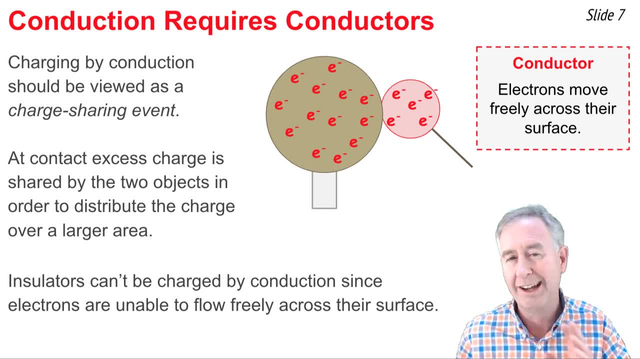 of electrons across their surface. So what would happen if you touched, say, a conductor to an insulator or an insulator to an insulator. What would happen then? Well, a number of things, And the first one is nothing could happen. But the second thing is that something could happen, And 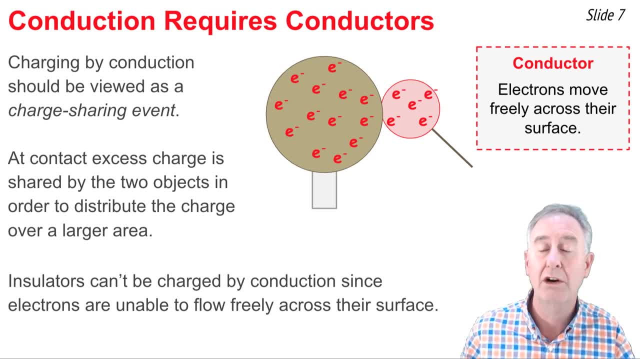 that covers it all there, And the something that could happen is that insulator could become charged by contact, by touching, but not this conduction process we've been talking about, by a process that I like to call charging by lightning. You'd hear a shock, You'd see a. 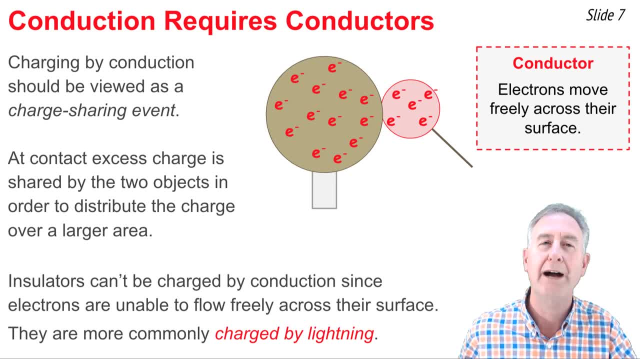 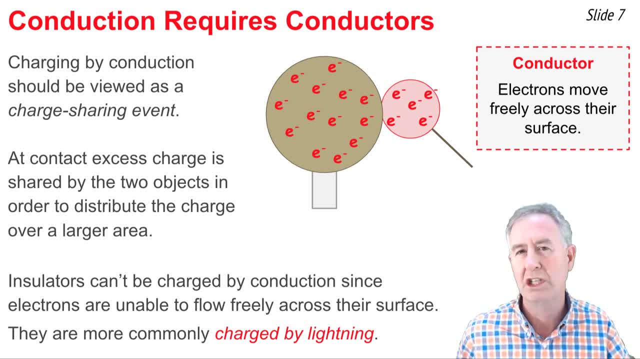 get an object really, really charged up and you touch it to an insulator And now all of a sudden air breaks down and becomes the conducting pathway through which charge jumps from one object to the other. And I refer to that as charging by lightning, But in general charging by conduction. 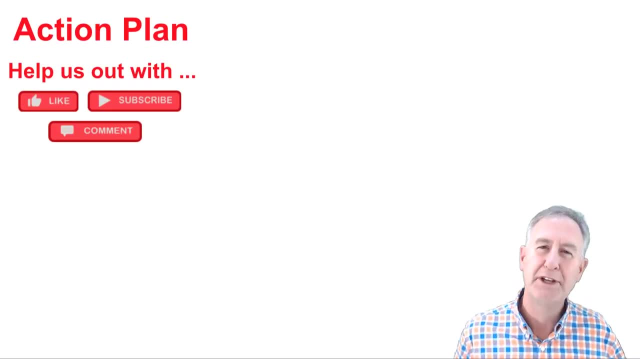 requires conductors. It's at this time in every video. I like to help you out with an action plan, a series of next steps for making the learning stick. But before I help you out, could you help us out by giving us a like or subscribing to the channel or leaving a question?